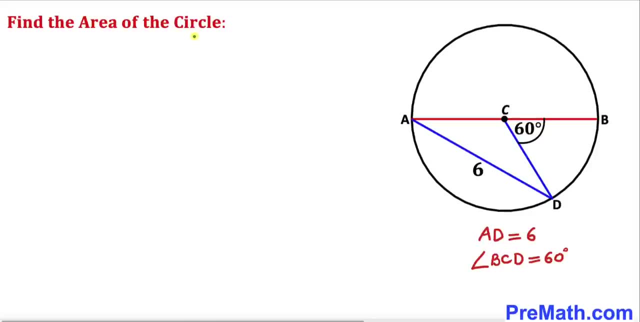 Welcome to PreMath. In this video, we are going to find the area of this given circle whose center is at C and this angle BCD is 60 degrees and, moreover, this chord AD is 6 units. Please don't forget to give a thumbs up and subscribe. So let's go ahead and get started. 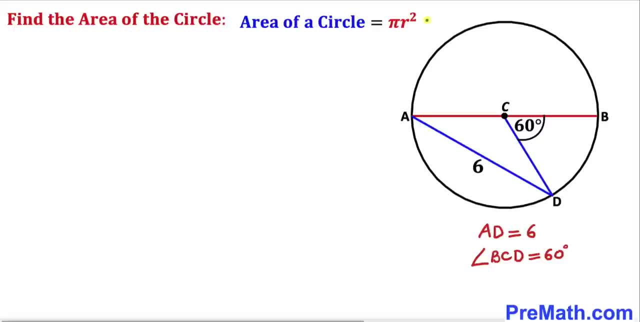 And now let's recall the area of a circle formula, which is pi r square, where r is the radius of this circle. So therefore, we are going to find the radius r of this circle and here r is the radius of this circle, as you can see. And now let's recall this central angle theorem. 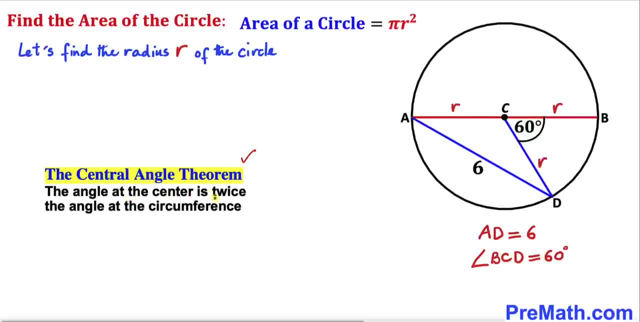 According to this theorem, the angle at the center is twice the angle at the circumference. We know that this angle at the center is 60 degrees and this is the angle at the circumference. Then, according to this theorem, this angle is going to be the half of. 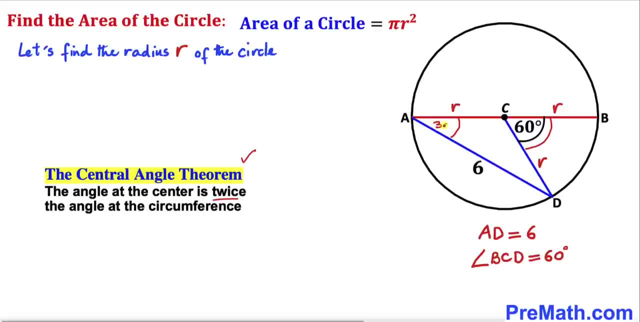 this 60 degrees, So that means this angle is going to be 30 degrees. So therefore, our angle CAD turns out to be 30 degrees, as you can see over here. And now let's focus on this triangle ACD. and we know that these sides- this side is r and this side is r as well. So therefore, this: 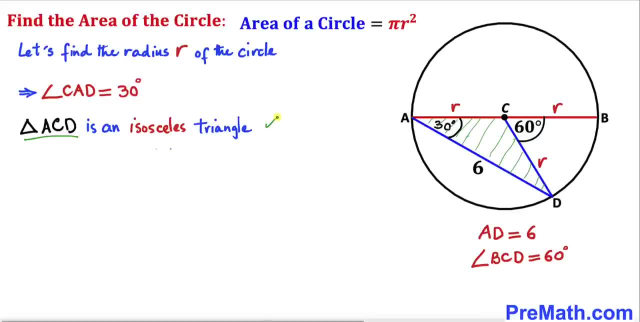 triangle. ACD is an isosceles triangle because this side length is equal to this side length. Here's our next step. Let's go ahead and draw a perpendicular from this point C onto this- uh, chord AD. since this perpendicular- so this has got to be 90 degrees- And since these two sides. 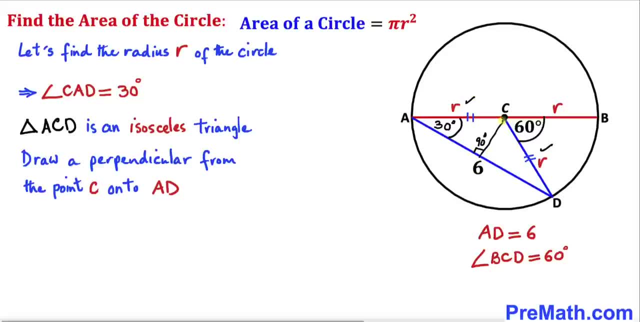 are congruent. so, therefore, this perpendicular is going to bisect this chord into two equal parts. This side is going to be this side. If this whole thing is six, then this is going to be three units, and this is going to be three units as well. So this is going to be three units as well. 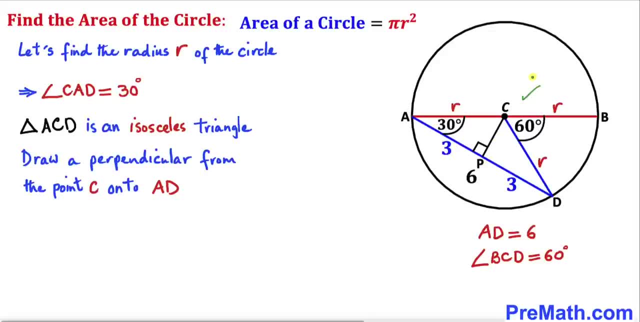 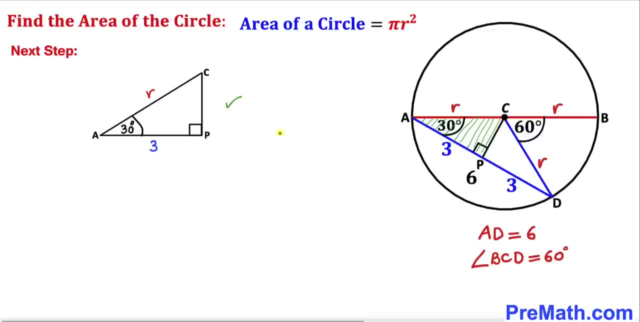 And here's our much nicer looking diagram. And now let's focus on this triangle APC, as you can see over here, And we can see that this triangle APC is a right triangle. And here I have copied down this right triangle APC, where this side length AC is radius r, this side length AP is three units and 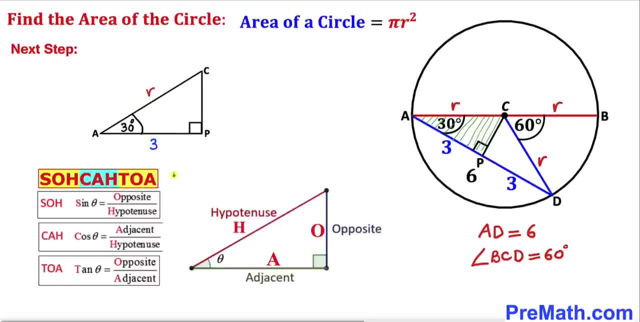 right angle is 30 degrees. And now let's recall this Soka-Toa chart and we can see that our cosine theta is equal to adjacent over hypotenuse. In our case, this side is our adjacent and this side is our hypotenuse. So therefore, our cosine of 30 degrees is going to be adjacent in our cases. 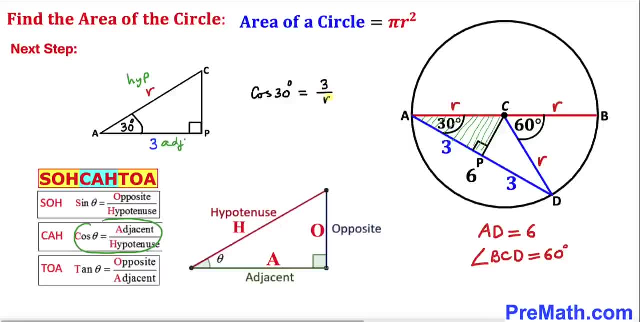 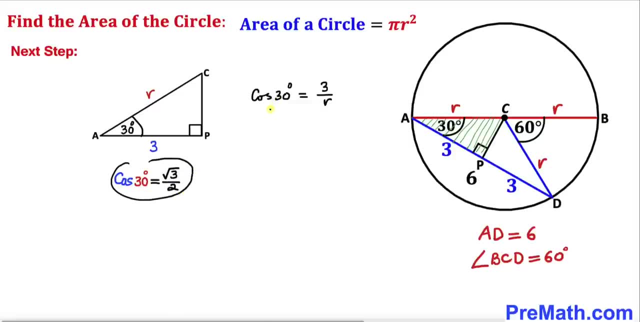 three divided by hypotenuse. Now let's go ahead and draw a perpendicular. So this triangle, APC is hypotenuse is radius r, and we know that cosine of 30 degrees is square root of 3 divided by 2. so therefore, i'm going to replace this thing, i'm going to write down square root of 3 divided by 2. 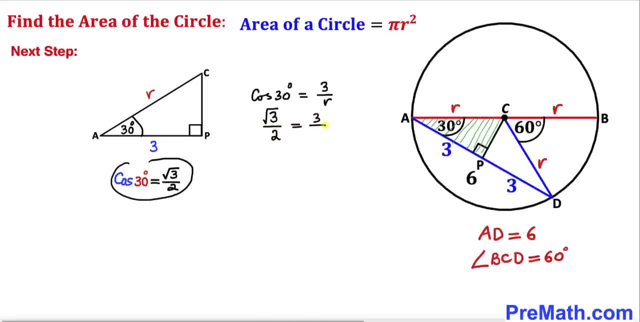 equals to 3 divided by r. now let's go ahead and cross multiply, so we are going to get square root of 3 times r, equal to 2 times 3 is going to be 6. now let's divide both side by square root of 3 to isolate radius r. this and this is gone. so radius r turns out to be 6 divided by. 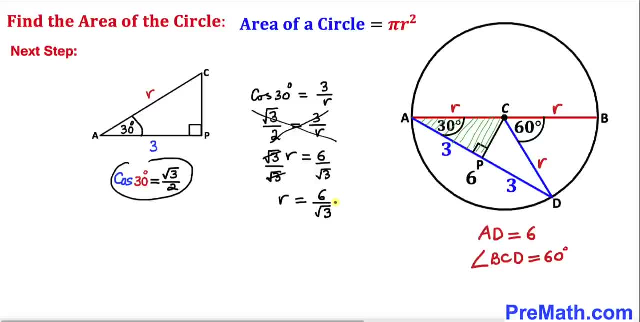 square root of 3. now let's go ahead and rationalize this part. i'm going to multiply and divide by square root of 3, so therefore our radius is going to be 6 times square root of 3. divided by this denominator is going to give us 3, and if we reduce this thing, our radius turns out to be 2 times square root of 3.